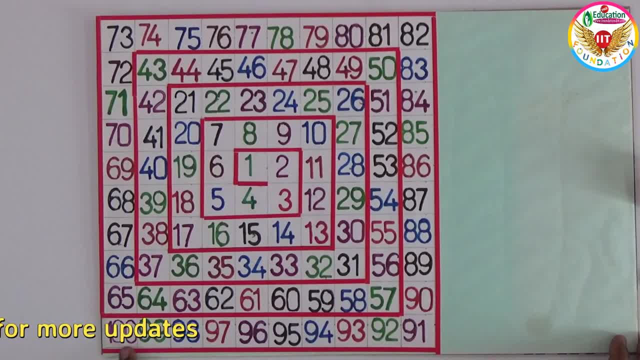 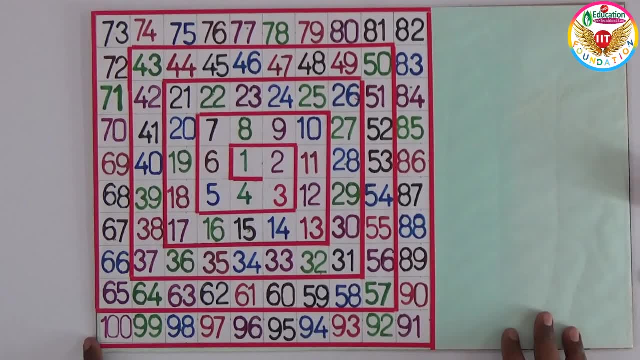 type So I arrange the numbers. You can see the clearly. so ending with 100.. So, along with this red color so you get the numbers are scrolling till to reach the 100. So we know the game that snakes and ladders right So we can get the chance. but apart from that, this is the game. 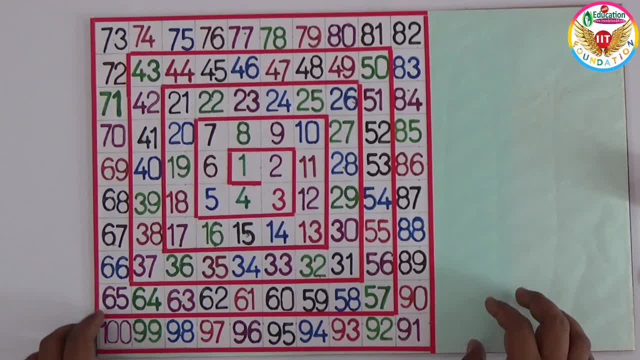 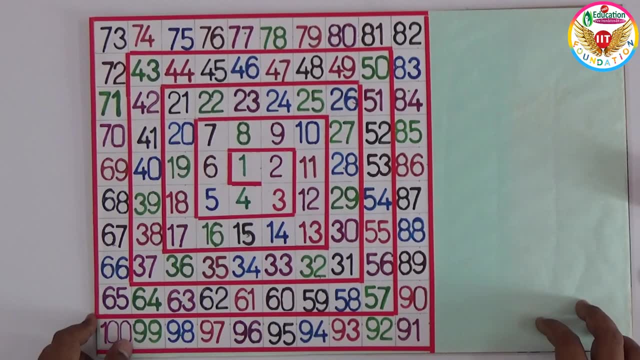 I prepared, with the based on the numbers to learn some simple concepts. For example, if you want to learn the multiples or even numbers, odd numbers, especially for child or children. those are the learning, the basics. we can play this in the game way like funny way. Oh, just only one example. I. 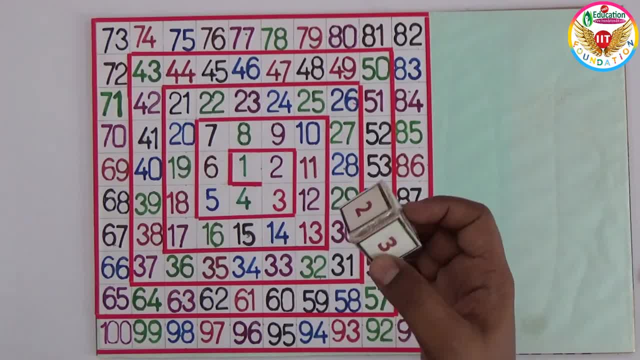 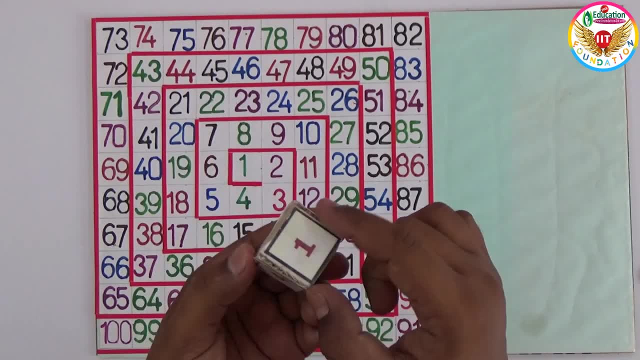 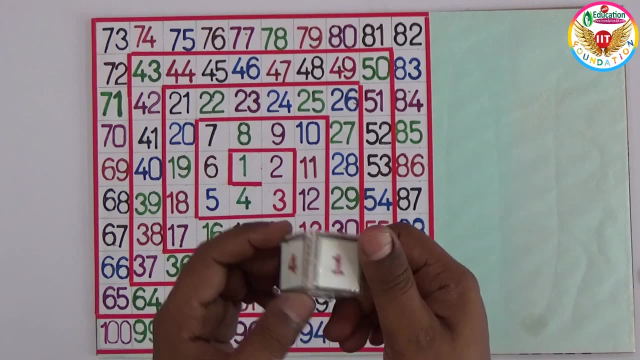 will show. Now we need one cube For this one dice. so is a cube shape, This one called dice. we can purchase from outside, also in the shops. but I prepared this. so I took the six pieces, six square boxes, six square shape things, and I prepared the box like this and arrange the numbers So we can play like this right. 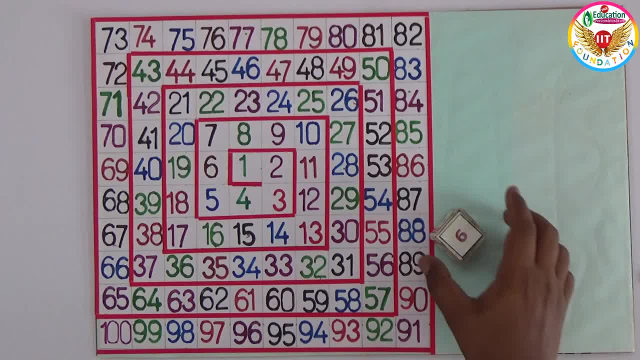 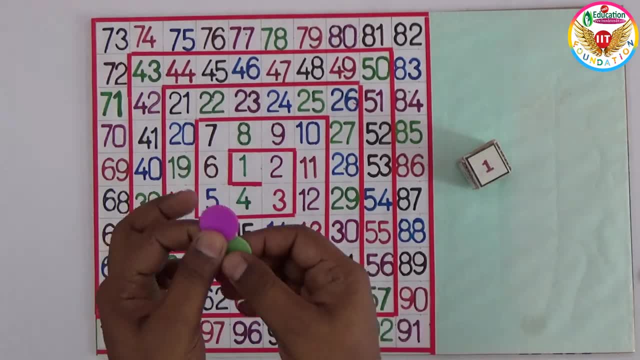 One, get the number Two. you can play six. So different, different, no chance to get one. So you can any number of people. you can play this this time taking two coins, For example, to make two coins. So you can make two coins. So you can make two coins. So you can make two coins. So 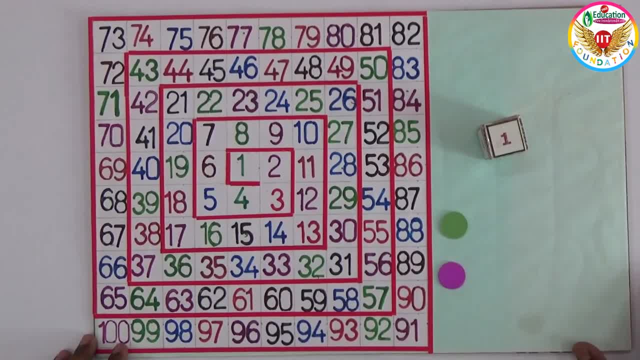 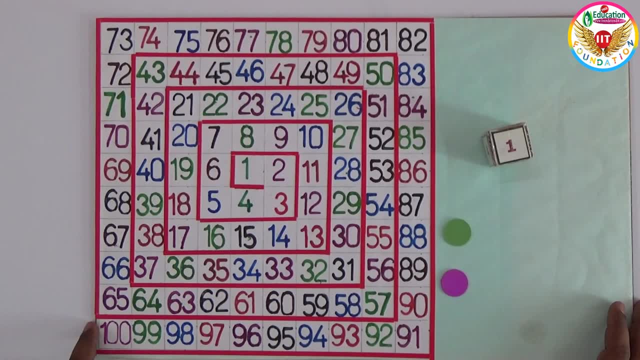 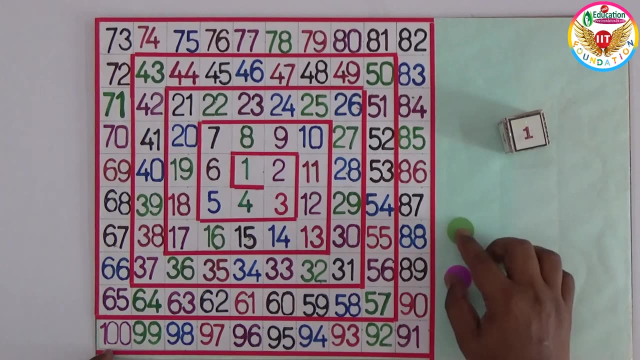 members are playing. now. one concept I'll explain. you can go in that way, remaining also, for example, if you want to learn the multiples of 4, multiples of 4 means 4, 8, 12. now, if you keep the concept, the learning of the multiples of 4, now the 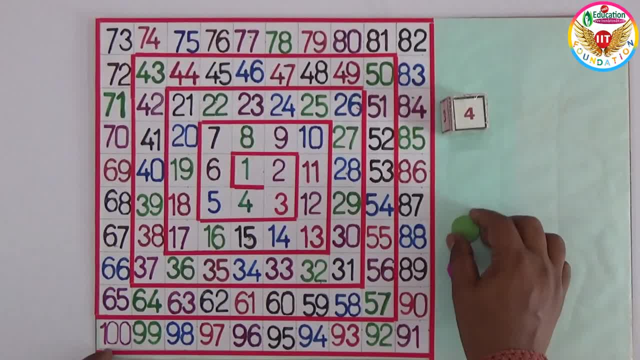 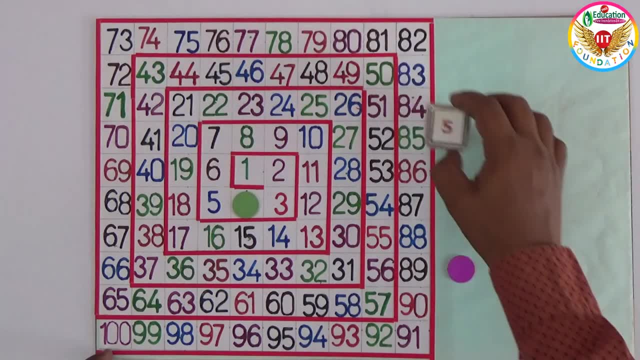 players should start playing, for example, first, when you got the 4. you'll keep 1, 2, 3, 4. who will get the multiple of that 4? you will play again second time. so you got the 5. that's why 1, 2, 3, 4, 5, 9- now it is not multiple of 4, so it is not. 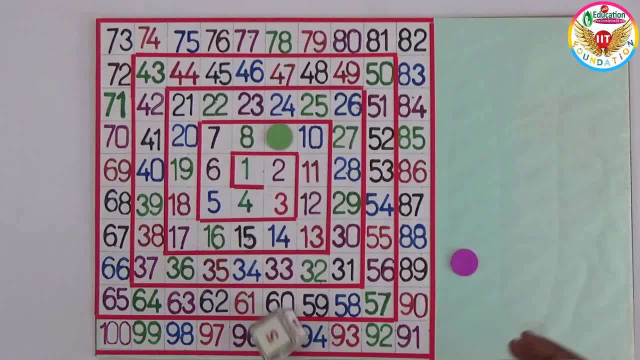 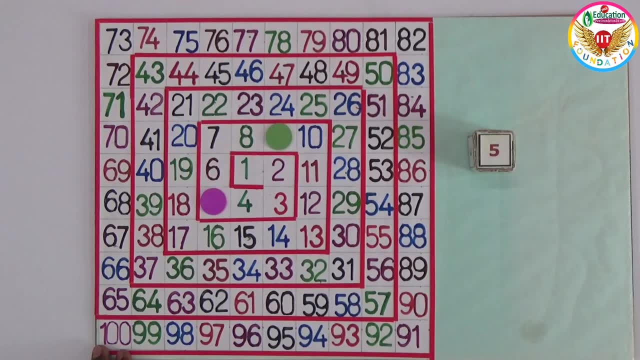 again. chance for second person. again, you'll play with one more. okay, got the 5, so 1, 2, 3, 4, 5, 5 is not multiple of the 4, so you'll not play again. once you get the multiple of 4, you need to roll the die again. okay, for example, now again: 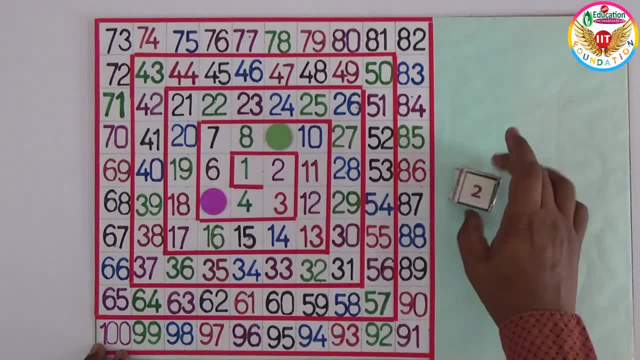 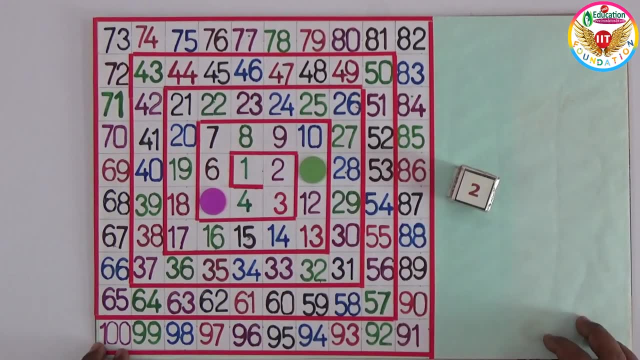 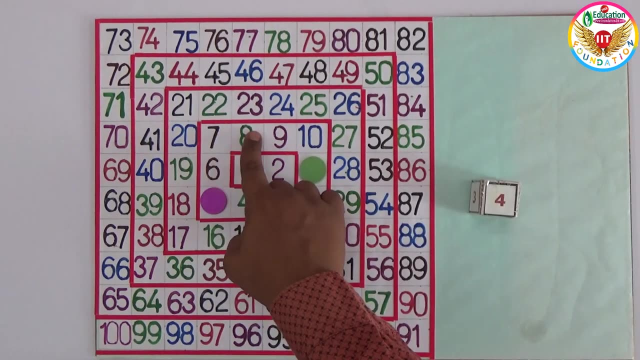 chance for first one, so you'll start with this 2. you got okay, 10, 11, so 1, 2. so already here. 1, 2 on the 11, so 11 is not multiple of 4, so you'll not play again, for the second person will start doing. you got the 4, so 1, 2, 3. 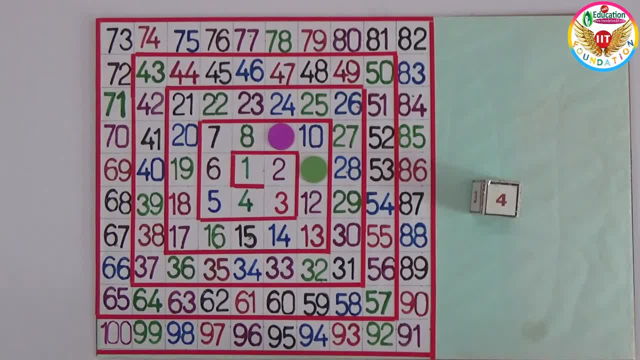 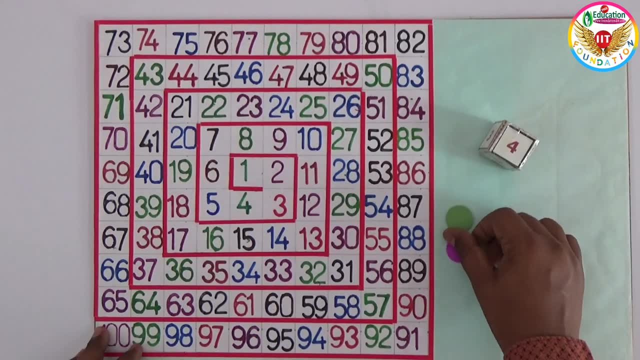 4, 9. so only when you get the multiple of 4 you'll play again. so we'll reach the hundred. first is the winner. not only multiple of 4, we can take the chance of multiple of 5, 6, 7, anything up to till 10. not only multiples, we can take some. 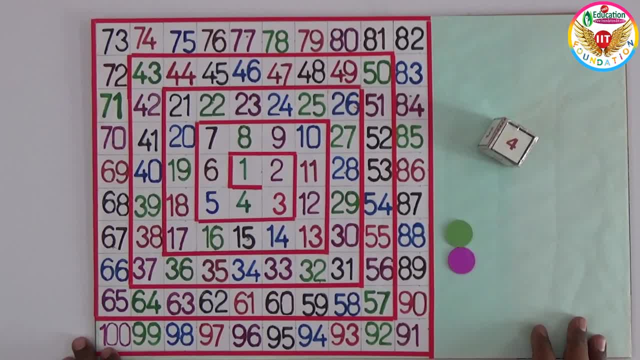 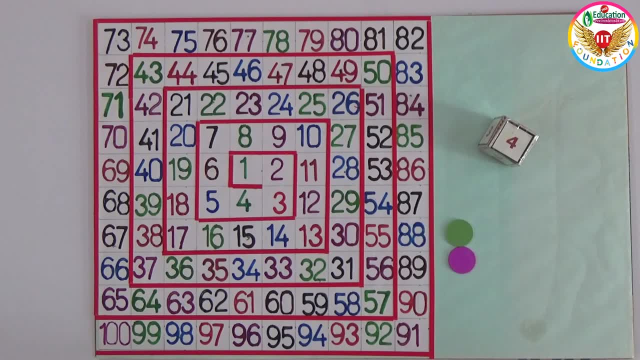 concept of factors, for example the factor cell for 20. so only 20 factor of factor to reach number 20. so again can take the odd number. so time number one person starts playing 3, 4, 1, 2, 3. get the number you need to play. 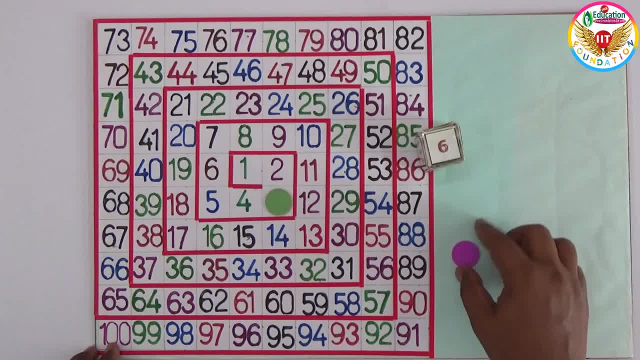 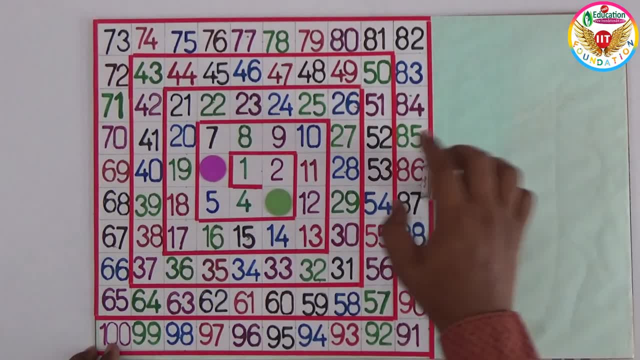 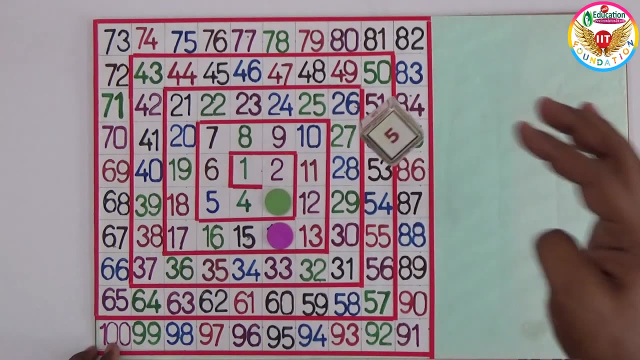 in to station ok. 1, 2, 3, 4, 5, 6, 6 is the even number number right. again you start playing 4, 10one 2, 3, 6, 4, 5, 6, four. you got even number. again you'll do again four. so these are chances until 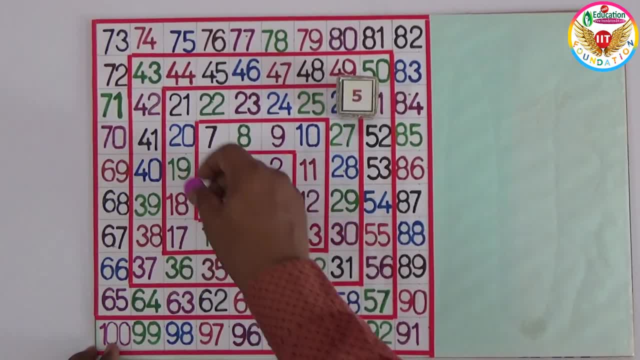 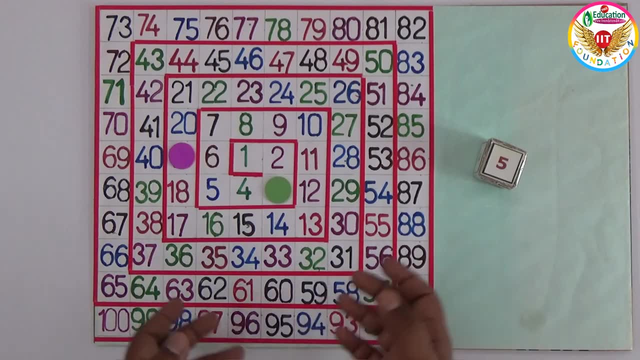 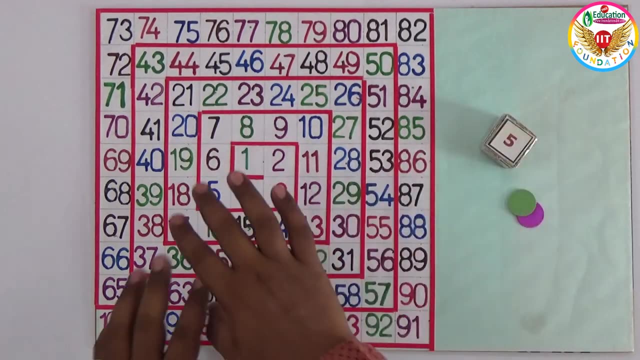 each no, five, one, two, three, four, five, so 19, so it's not even number. again, chance per second right. so this the funny way, and by learning some simple concepts in maths, we can use this spiral board number game, so only need some dice and you can add in the numbers in this way and you can play. so the multiples of any. 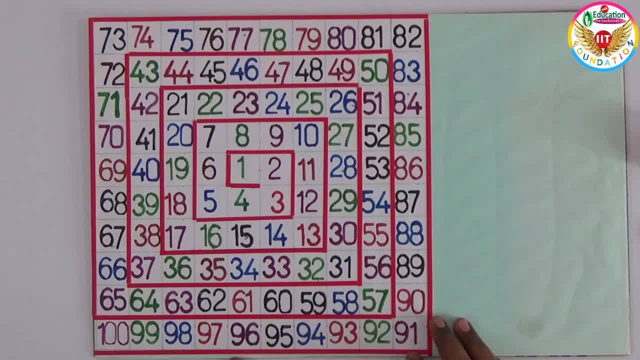 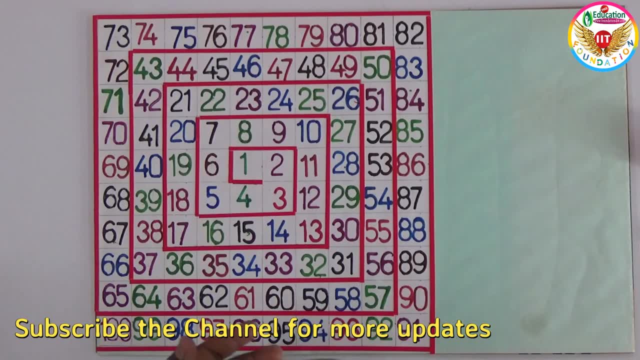 numbers, some factors, even numbers. even you can take the concept of prime numbers also. so we'll get the prime number, will play again. so that means they can understand what is the different different situations by meanwhile, by playing, their learning right. so that's why they never forget. 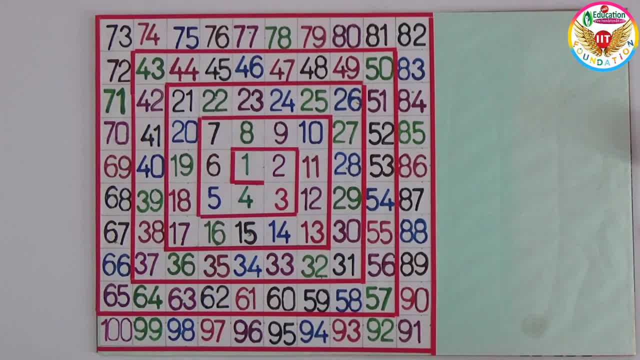 so this is simple and easiest way to learn some simple basic concepts. so this is the project.